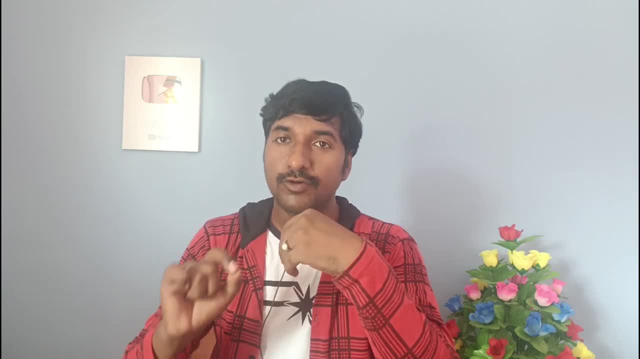 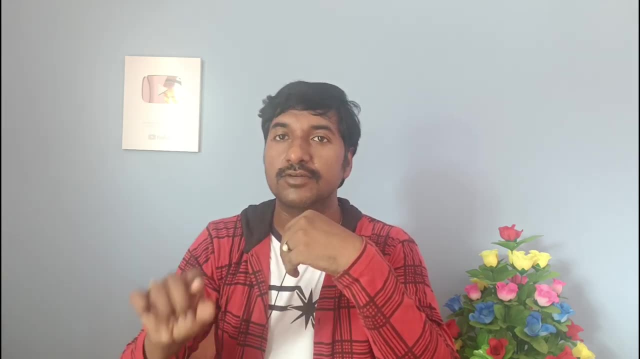 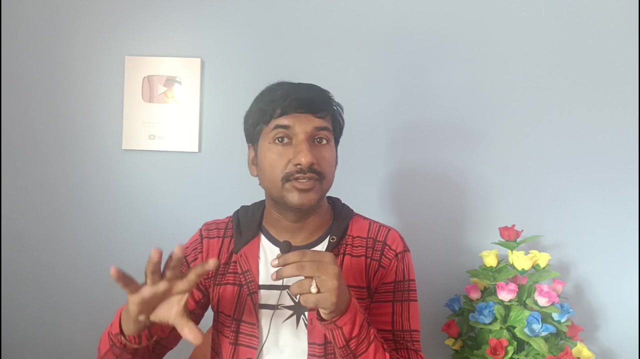 within a large device or machines. Let me tell you one of the best example. then everyone can understand, and nowadays everyone using in their homes as well. That is nothing but washing machine. In that washing machine some small computer is existed that controls the operations of the 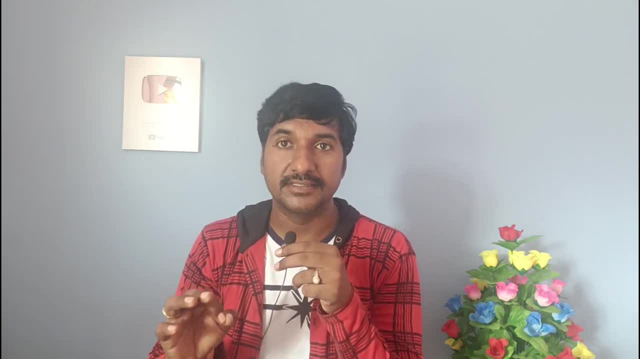 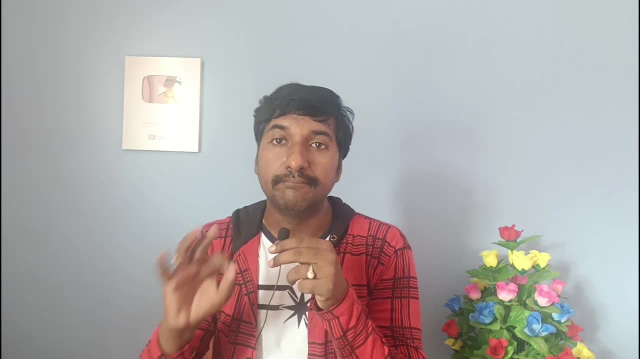 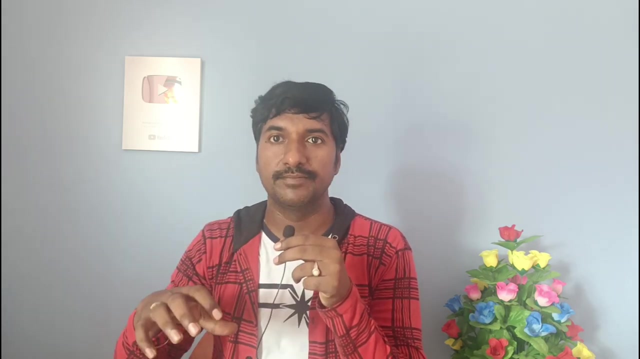 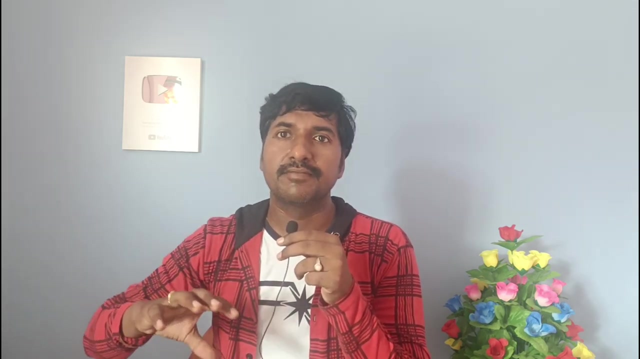 washing machine, such as controlling the water temperature, washing cycle and spinning the drum, So that small computer is nothing but an Embedding System Like this. there are many furnitures, many devices are there in our home only like microwave, okay, and washing machine and refrigerator. So like this, there are many devices we are 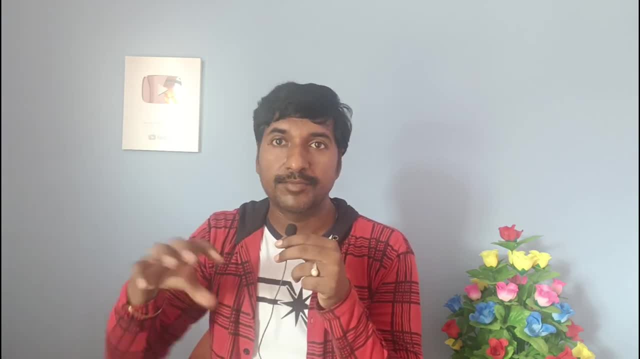 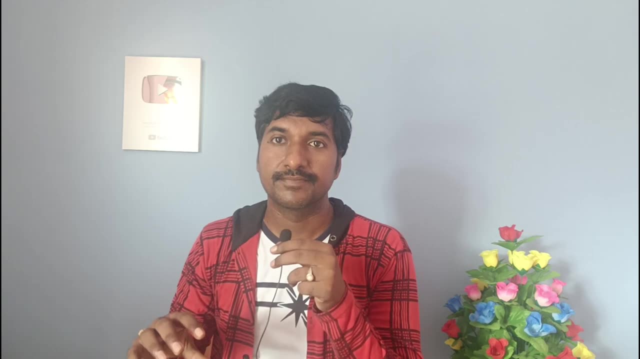 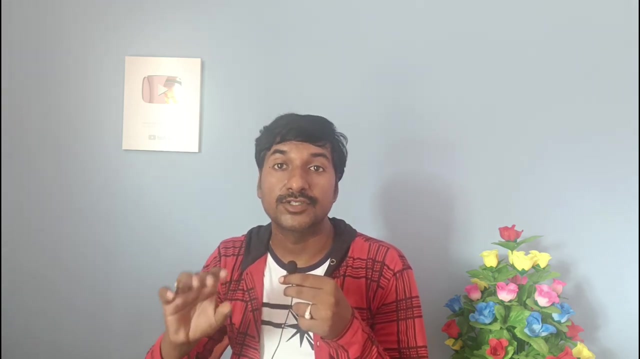 using in everyday's life. Even we can see these type of Embedding Systems in the modern cars, microwaves, microwaves and medical devices, digital cameras, and in our household things as well. Let us start. As I already told you, Embedding System Engineers works with the combination of hardware and 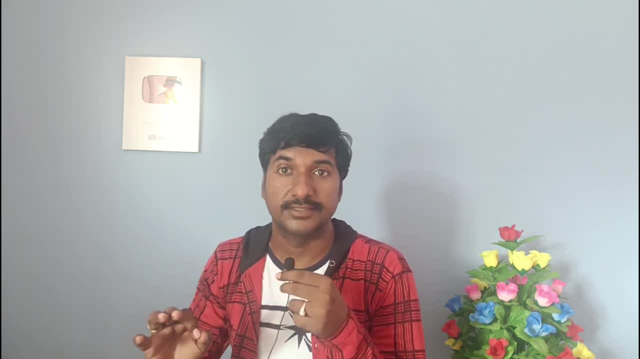 software to perform a particular task or functions. They are responsible for selecting appropriate hardware components, such as microcontrollers or processor, and developing the software that controls or interacts with the components. So you may have doubt in which industries are mostly used these kind of projects. So 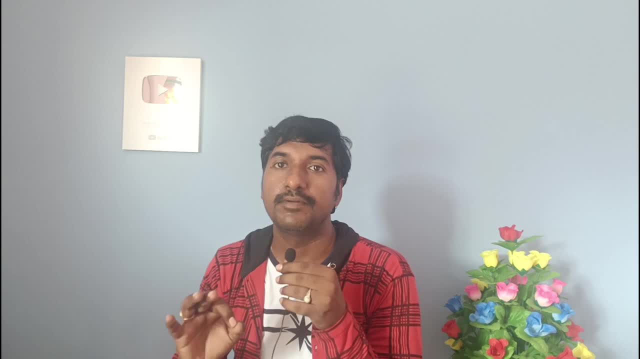 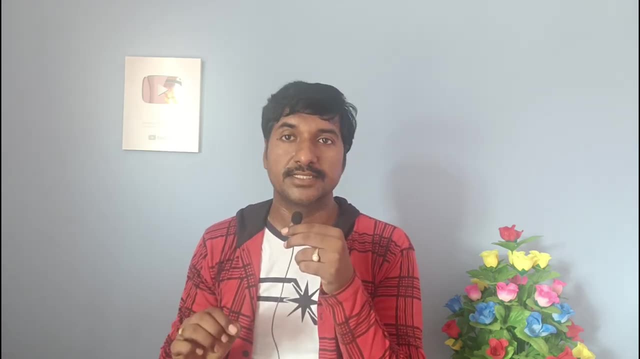 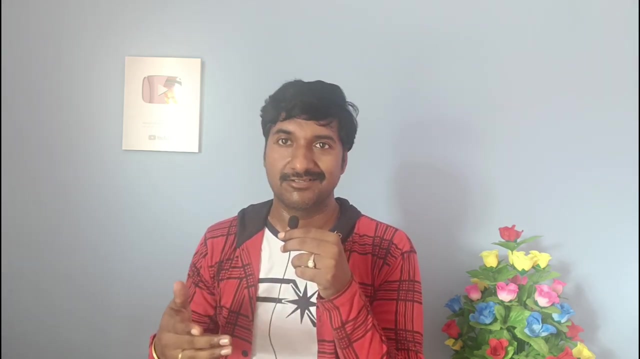 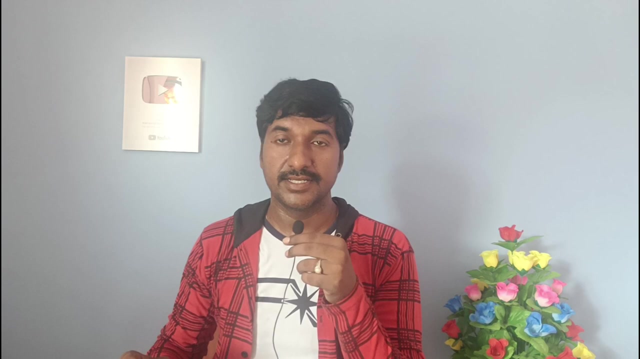 let me tell you few popular industries where most of the projects are using MBD system engineers, such as Automative App, Aerospace and in mobile device as well, and circuit design. and consumer electronics as well, and the IoT device as well, industry automation as well, and medical devices as well. So, like these, we are using these. kinds of projects in widelange of industries. So though, an additions for an Embedding Systems. so for an example you can see here, Let me translate that for me and I will show how an Embedding systems are organized in a washed floor. Let me tell you few. let me tell you few popular industries. 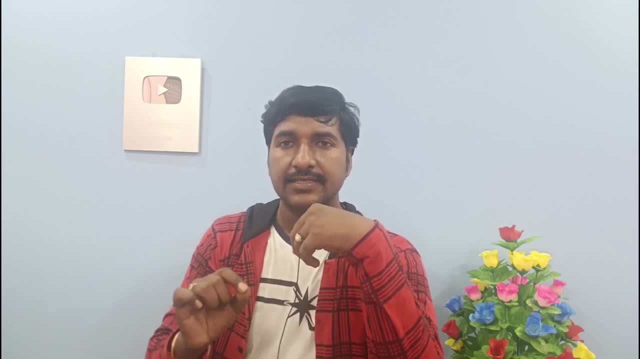 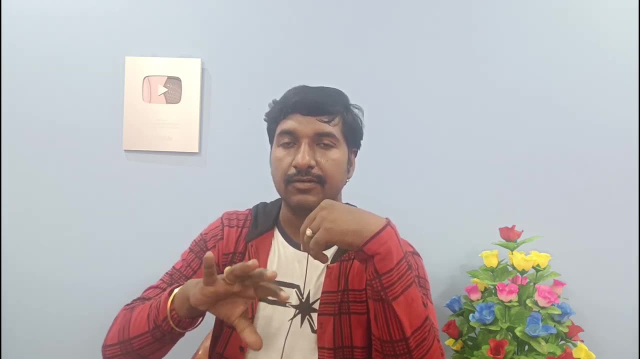 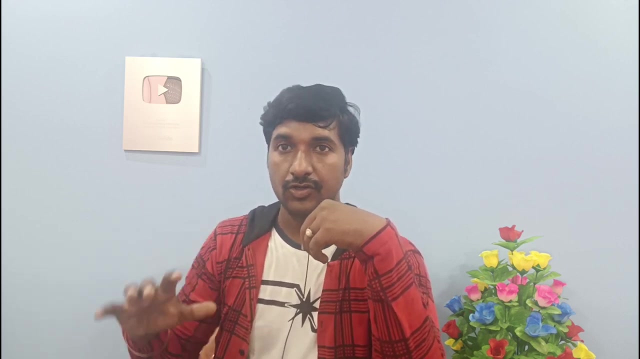 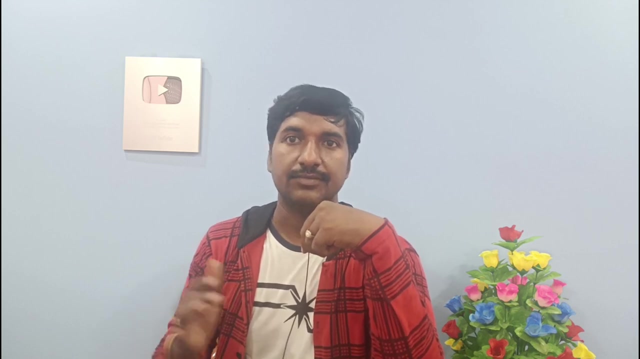 in wide range of industries, guys. i can say in simple statement: you can use these type of systems from small device like micro ovens to complex systems like industrial automation, industrial control, automation device. okay, another question is: what type of skills are required to become a embedded system engineer? so you must be strong in programming skills, guys. so 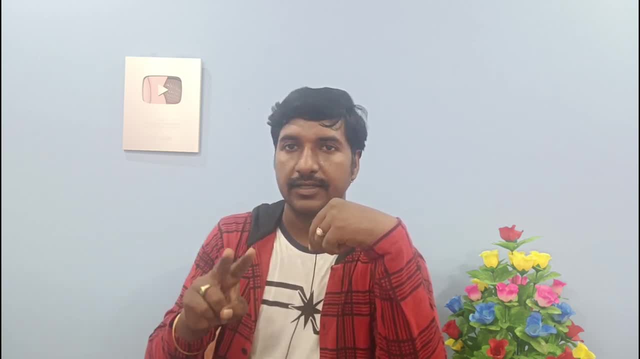 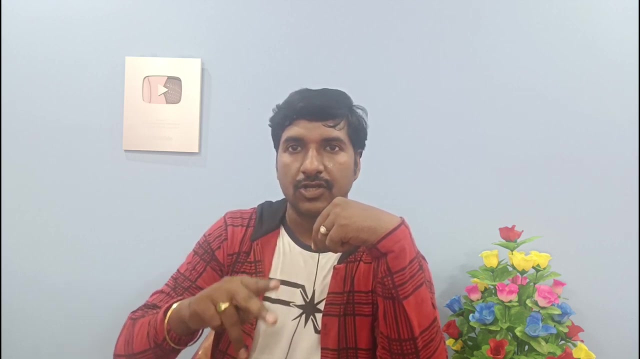 those programming skills are nothing but either c or c++. i highly recommend you. you must be strong in c programming language, with data structures okay. and second one is: you must be good at not only software, you must be good at hardware skills as well, like circuit design. 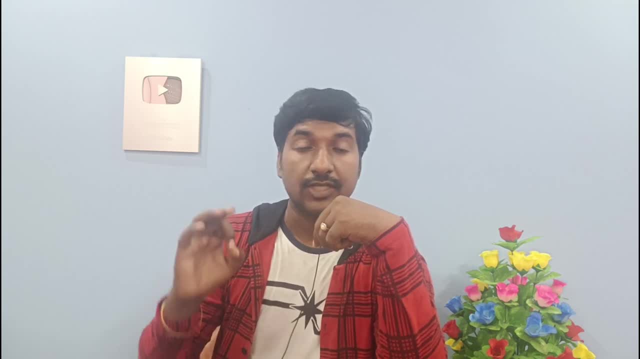 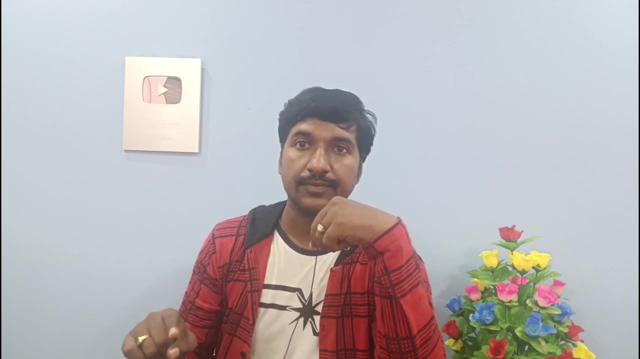 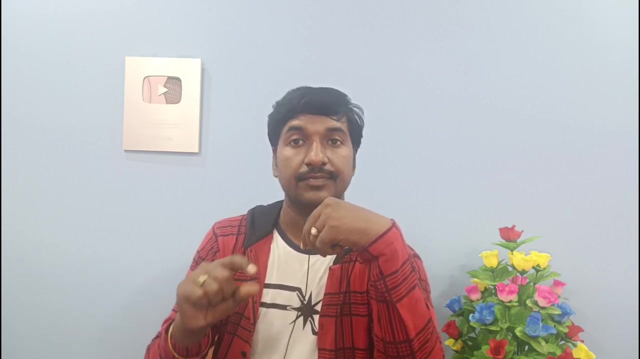 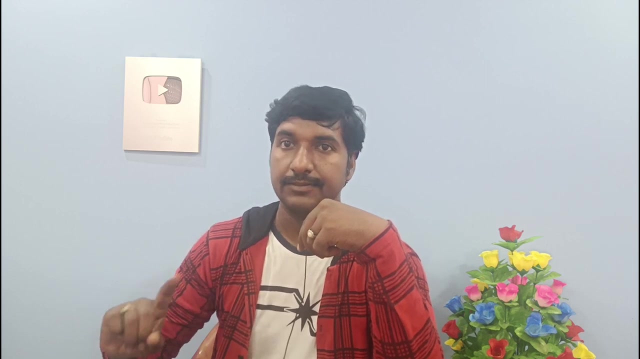 microcontroller, electronics, circuit design and digital signal processing, real-time operating system, rtos, communication protocols and debugging skills and testing skills as well. here you must be familiar with microcontrollers such as arduino, rossberry pi or arm based processor, and also as a embedded system engineer, you should have understand. 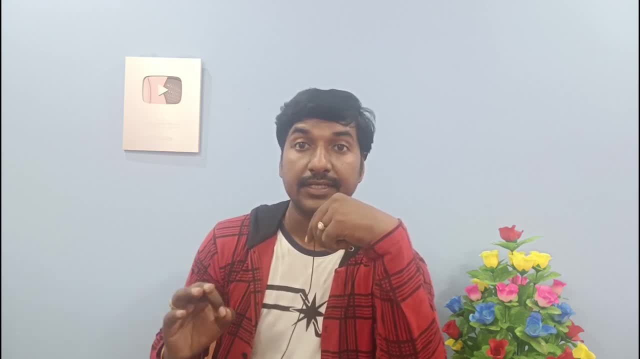 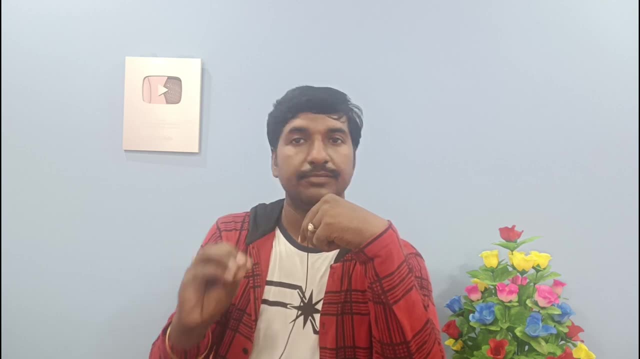 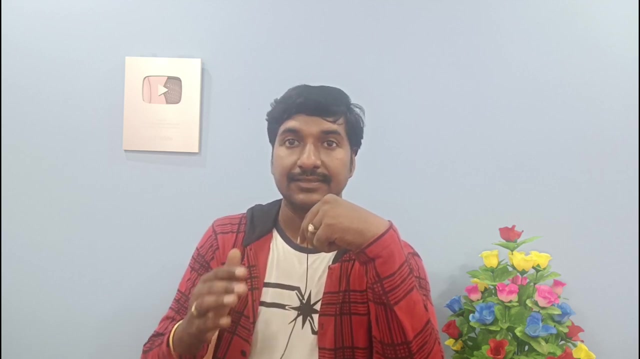 how to use microcontrollers and how to use microcontrollers and how to use microcontrollers, manage task scheduling, interrupts and memory constraints in embedding systems. if you have good knowledge or experience on the skills, then you definitely become a embedded system engineer. and apart from those skills, you must be stay updated with our latest trending technologies. 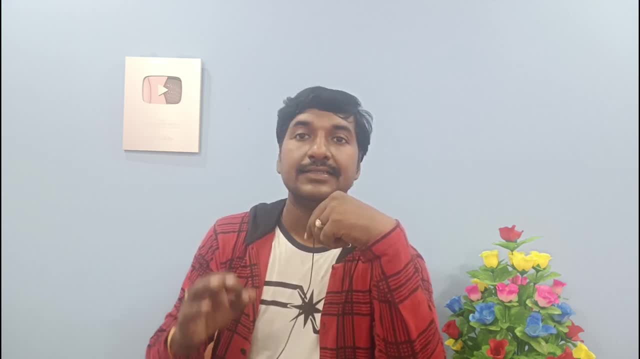 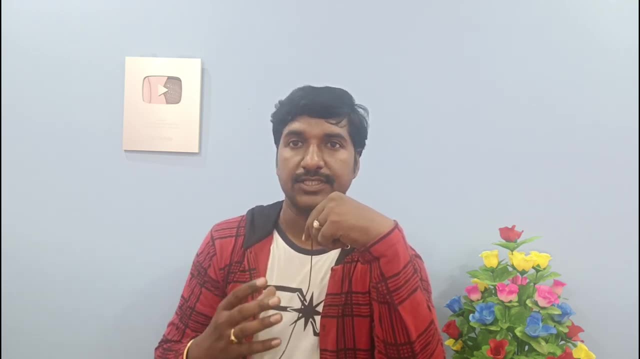 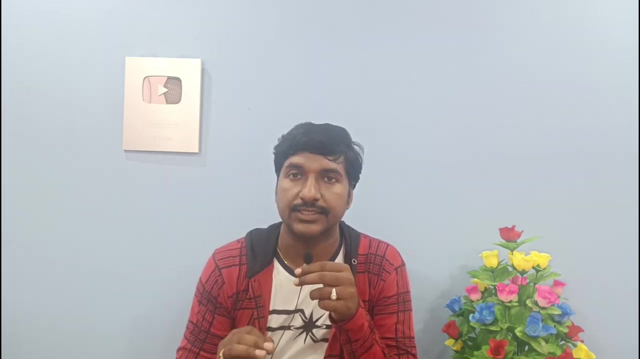 as well. guys like a wireless communication, uo t and cyber security related uh technology as well. now let us talk about what is the career scope of our embedded system engineer. embedded system engineers are in demand for designing innovative product, improving existing systems, ensuring efficient and reliable operation. you can find these jobs in number of industries like consumer electronics, like healthcare, aerospace, like iot device and cyber security related jobs, industrial automation and automobile automation device. find a number of job opportunities on these industries, guys. so not only in this industry, there are many industries are there. we can find number of job opportunities, uh, with this embedded system engineer. okay, now let me tell you what is the average value for this job role. if you are a entry level candidate, you will get between 3 lakhs to 5 lakhs for nm guys. so if you are a mid-level mb system engineer and if you have 5 to 8 years of experience, then you can find. then you will get like 7 lakhs to up to 15. 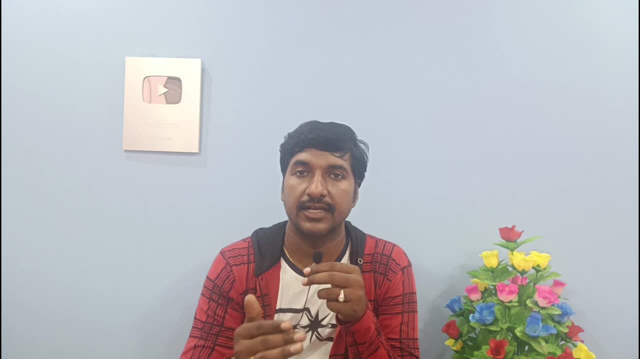 lakhs for nm guys. so for talking about the, then you can dem prestige you are looking to be a professional in, you can also get good pay, as mentioned. let me tell you right now. so you have a better pay cheque that you set for yourself. guys, it completely depends on your. skill set and whatever company you are looking for, whatever company you are applying for, if it is a broad based company and good company, then you can expect up to 20 lakhs for nm for eight years of experience. candid guys, okay. finally, my concluding words are: it's: 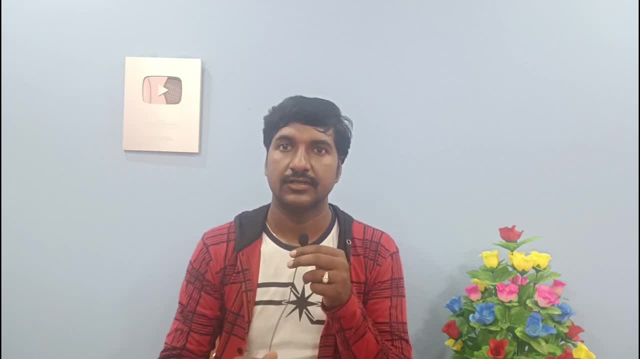 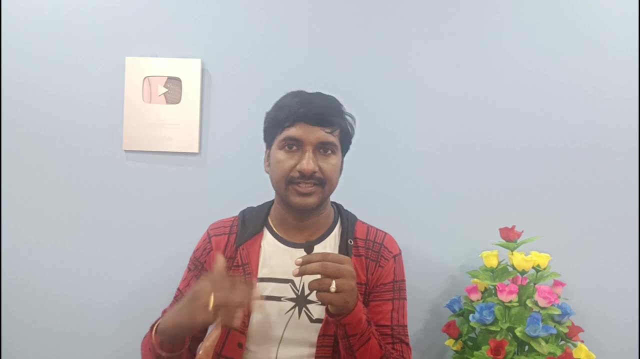 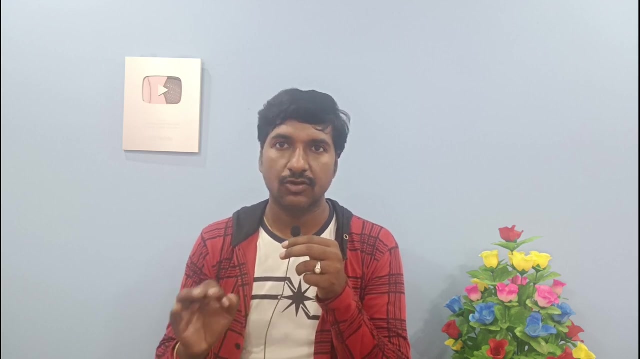 it's always strong network as well which are relevant your skills. so that's all, guys, for this session. I hope you enjoyed a lot for this session and you cleared all your doubts related to embedded system engineer job scope and career okay. so if you still have any doubts, please comment in the comment section. I will reply to.